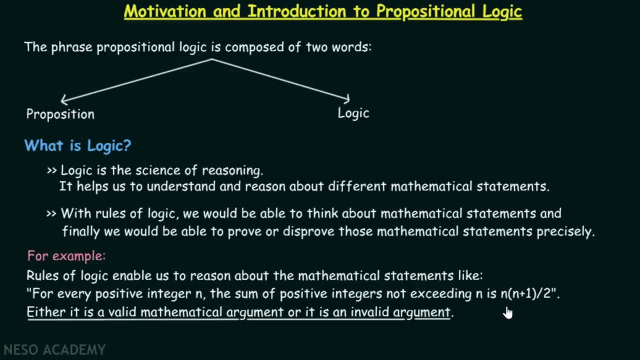 Which is nothing but the sum of first n natural numbers or sum of first n positive integers. Right, So this particular mathematical statement is a valid mathematical statement And we would be able to prove this particular statement with rules of logic. Either it is a valid mathematical argument or it is an invalid mathematical argument. 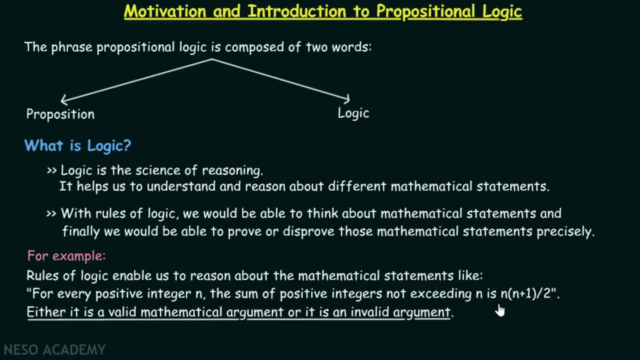 But we know that this mathematical argument is a valid mathematical argument, And we can prove this also with the help of logic. This is what a logic is all about. With logic, we would be able to reason about statements. We would be able to think about mathematical statements. 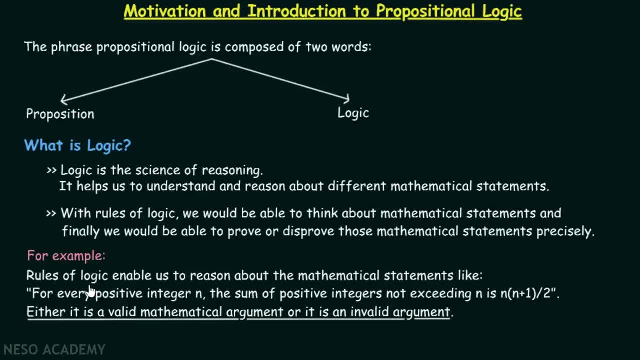 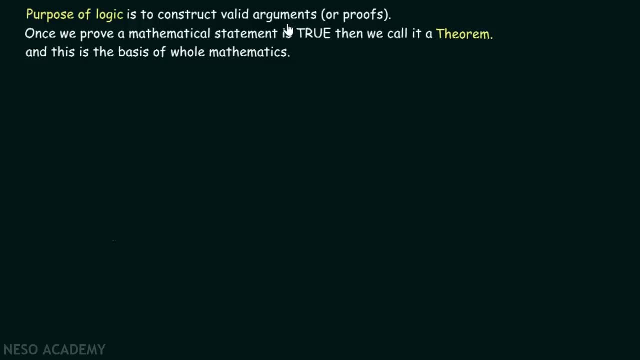 And, finally, we would be able to prove them or disprove them by using certain rules that are provided by logic itself. Now let's try to understand what is the purpose of logic. Purpose of logic is to construct valid arguments, First of all. this is a very important point to note. 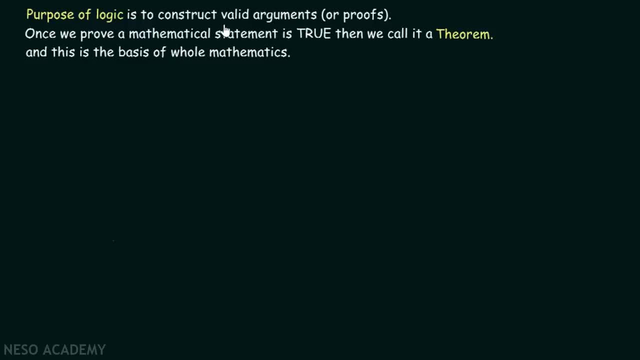 This is already. we know that purpose of logic is to construct valid arguments, Valid arguments, which are also called as proofs. Once we prove a mathematical statement is true, then we call it a theorem. We already know that When we prove a mathematical statement is true, 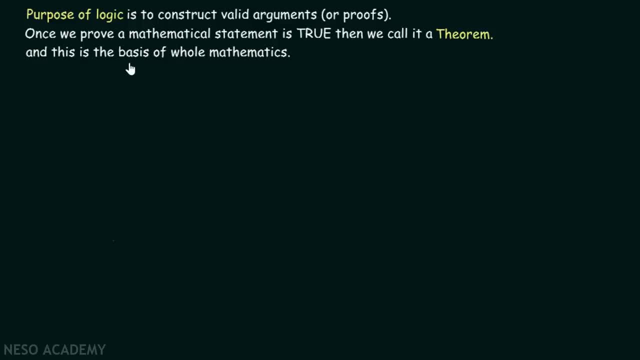 then we call it a theorem, And this is the basis of whole mathematics. Right, This is the basis of whole mathematics. Therefore, logic is very, very important. Let's consider one more example Here. in this example, we are talking about one famous puzzle. 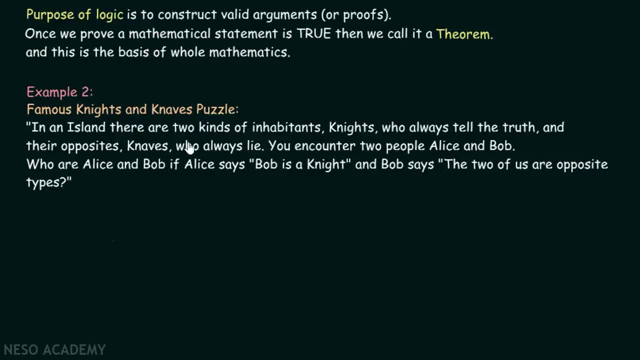 called Knights and Knaves puzzle. In an island there are two kinds of inhabitants: Knights, who always tell the truth, and their opposites, Knaves, who always lie. You encounter two people, Alice and Bob. Who are Alice and Bob? If Alice says Bob is a knight? 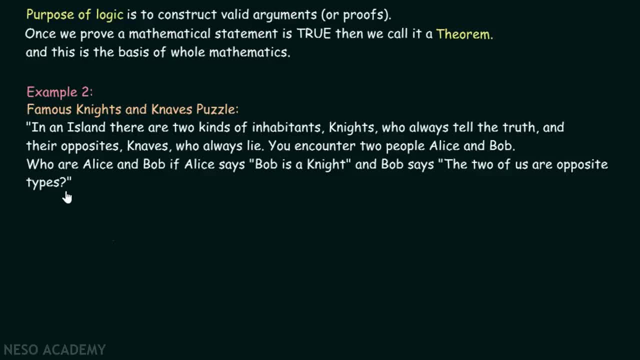 and Bob says the two of us are opposite types. We want to know that. who are Alice and Bob? If Alice says that Bob is a knight and Bob says two of us are opposite types? These kinds of puzzles we would be able to solve very easily. 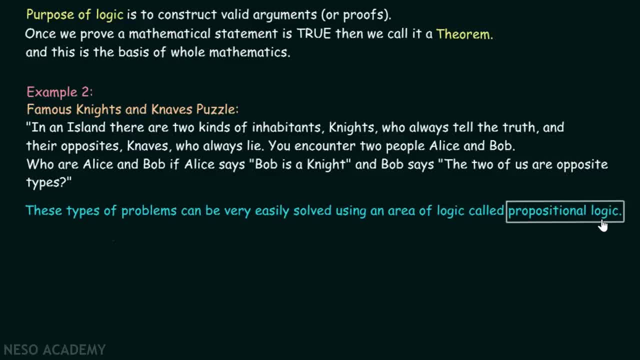 using an area of logic called prepositional logic. Please note down: With prepositional logic, we would be able to solve these types of puzzles very easily and in a systematic manner. That is the application of prepositional logic. Therefore, learning prepositional logic. 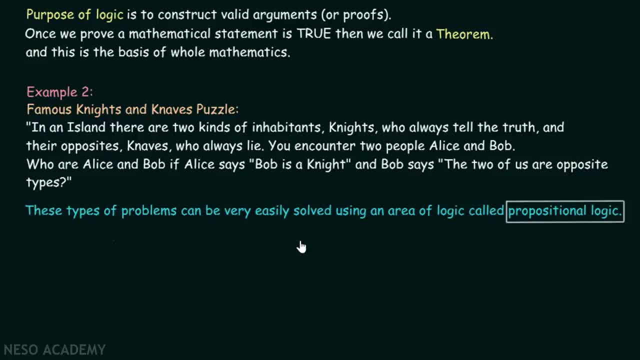 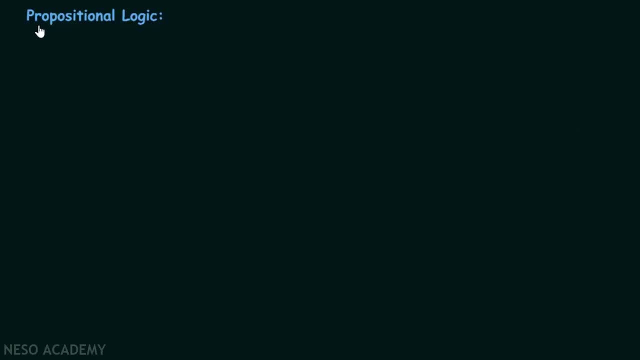 is fun and is very important. Now let's try to understand what is prepositional logic. We already know that prepositional logic is an area of logic, But in order to understand what is prepositional logic, we need to understand what is preposition. 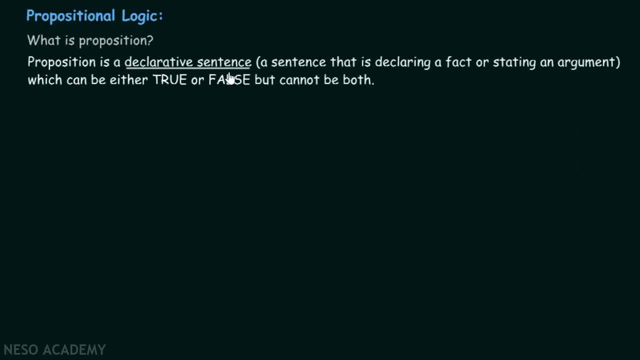 Preposition is a declarative sentence. Please note down: Preposition is a declarative sentence. Declarative sentence is a sentence that is declaring a fact or stating an argument, which can be either true or false, but cannot be both. Please note down this point. 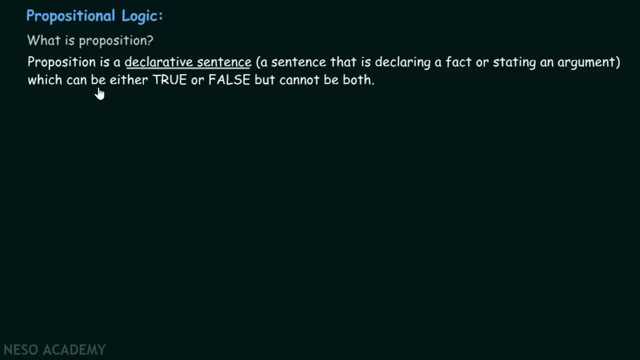 Preposition is a declarative sentence which can be either true or false, but it cannot be both. For example, Delhi is the capital of India. It can be true or it can be false. Water froze this morning. Definitely, this statement can be true or false. 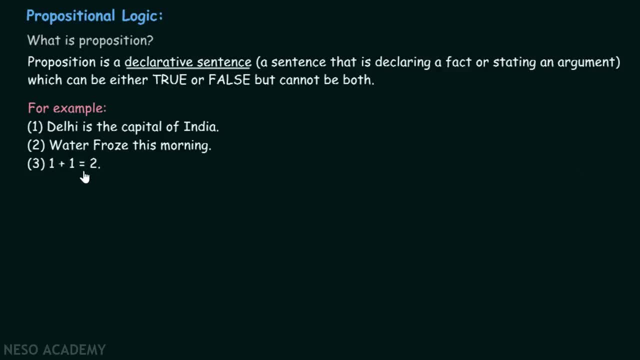 One plus one equals to two. We know that this statement is true. Also, it is a declarative sentence. Therefore, this is a preposition. Now let's consider some more sentences which are not prepositions. What time is it? 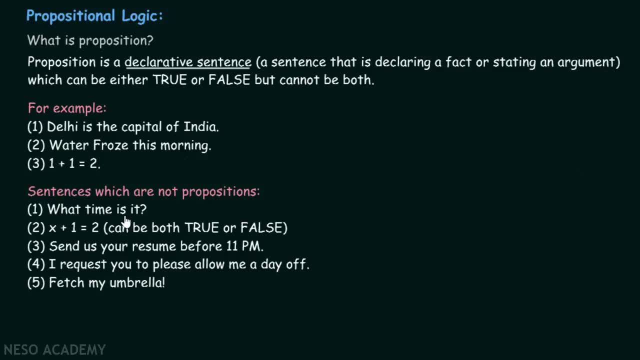 This is not a preposition, because this is not a declarative sentence. It is asking something: What time is it? It is not declaring a fact. Therefore it is not a preposition. X plus one equals two. It might seem like it is a declarative sentence. 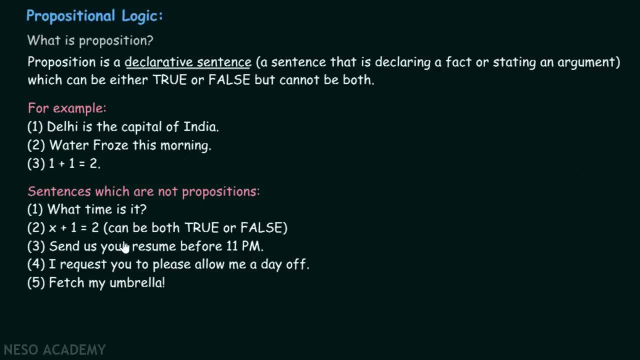 But think about it. It can be both true or false. Maybe you provide x equals to one. In that case this statement is true, But if you provide x equals to two, then this statement is false. Therefore, we are not certain about this statement. 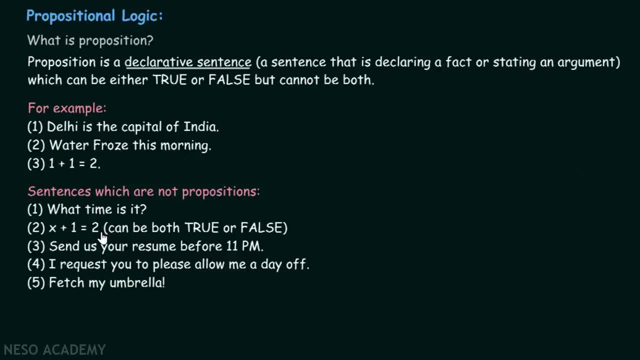 It totally depends on the value of x. Therefore, we cannot say that it is a preposition. As we know, preposition is a declarative sentence. that can be true or false, But it cannot be both. Send us your resume before 11 pm.